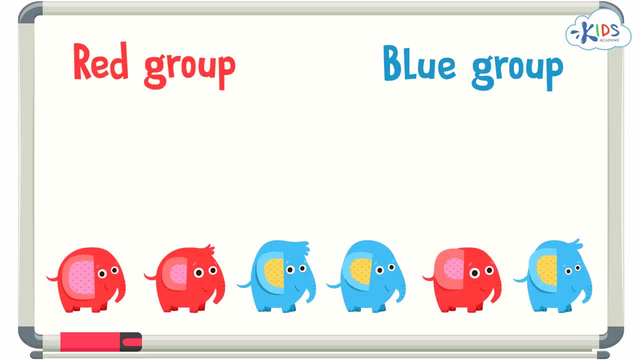 how to sort these objects, and we can start with the first object. In this case, we are sorting these super cool elephants. They are my favorite animal. If we look at the name of the groups, we can see that we are sorting by color and we will. 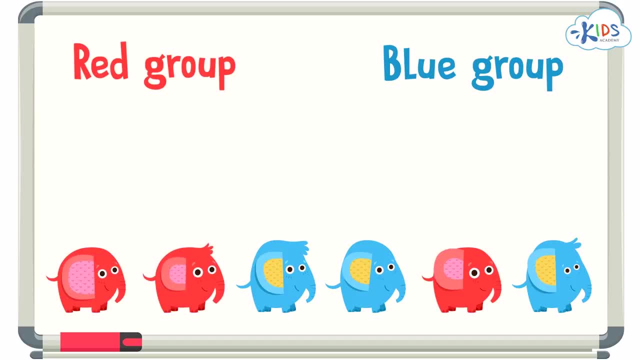 put the blue elephants on this side and the red elephants on this side. Let's take a look at our elephants and start sorting them into these two groups. The first elephant belongs in the red group. It's a red elephant. The next elephant belongs in the red group too. 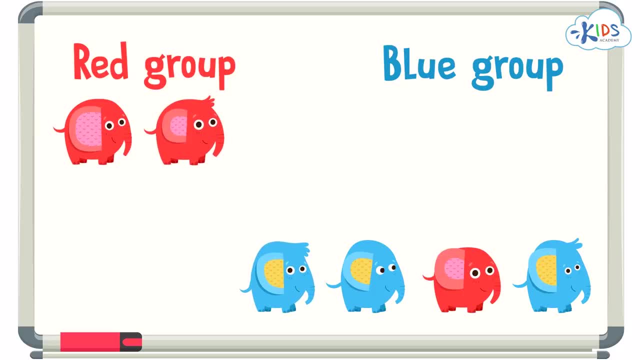 It's also a red elephant, But check it out. The next elephant is blue. This elephant belongs in the blue group because it's a blue elephant. The next elephant also belongs in the blue group. It's a blue elephant too. This elephant is red. 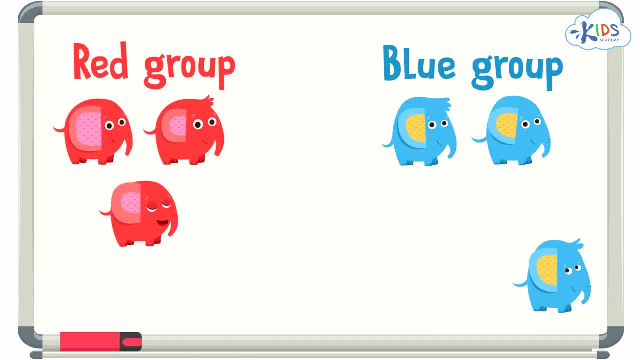 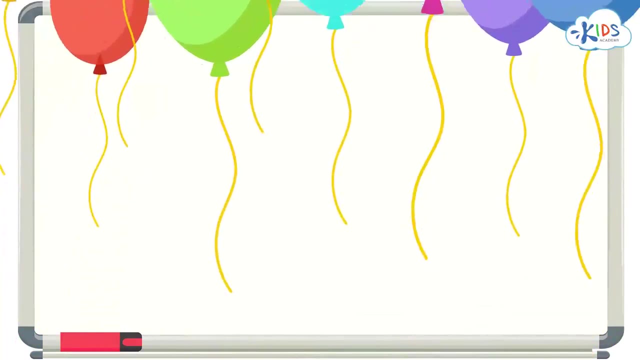 belongs in the red group: It's a red elephant. The last elephant belongs in the blue group. It's a blue elephant. Now we've sorted all the elephants into two groups. Sweet, Let's try to sort one more group of objects. We'll get started. 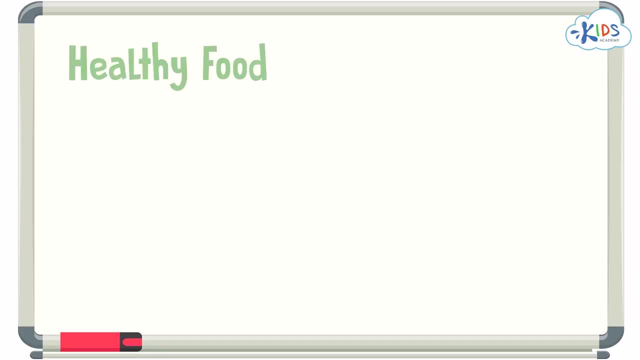 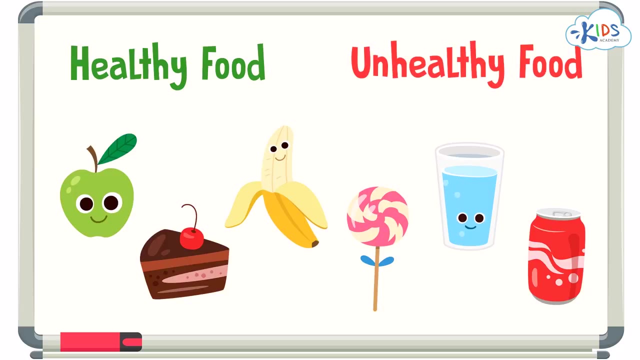 together, but I'll ask you to finish sorting these objects on your own during challenge time. This time the groups will be different, so I'll have to pay close attention to detail. Let's take a look at our new objects and the groups we'll. 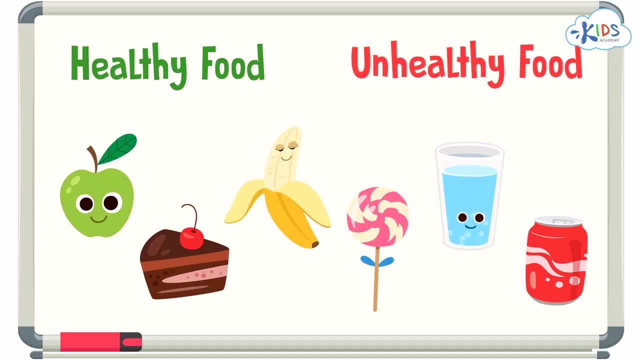 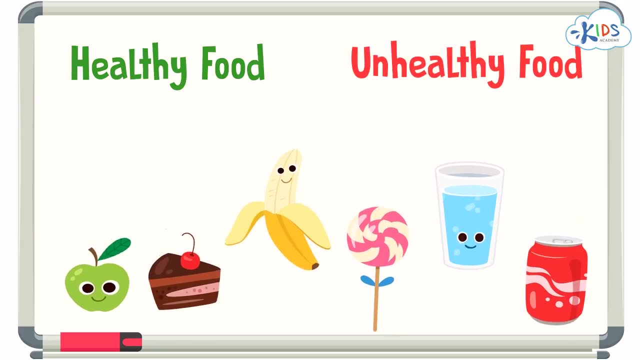 be sorting them into. It looks like we have some food. The names of the groups are healthy food and unhealthy food. We'll take a look at the objects one by one, and then we'll have to decide if it's a healthy piece of food or an. 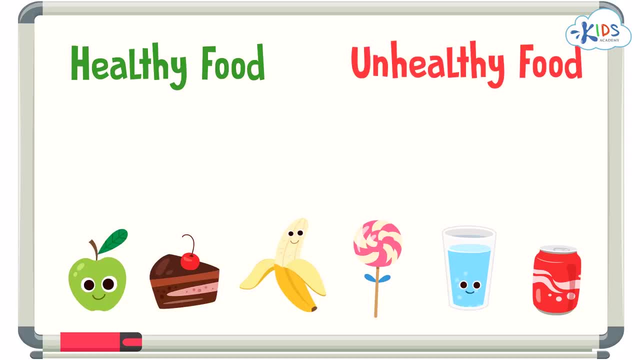 unhealthy piece of food. Let's get started. This is an apple. I know that apples are healthy and good for you, so let's get started. Let's put it in a healthy food group. Now we have a piece of cake. It sure looks yummy, but even though it's tasty, it's definitely unhealthy. Let's